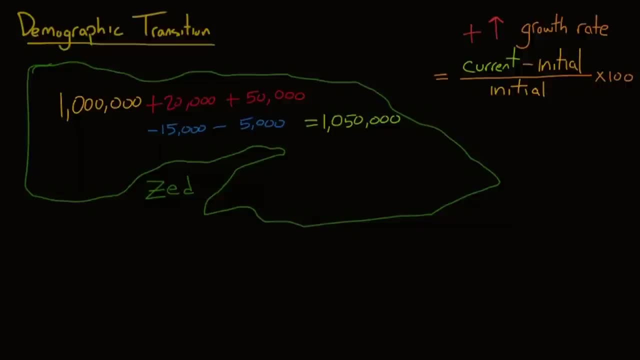 Now you have your growth rate. So now you can see why. when we say there's a positive growth rate, that means that the population is now bigger than the population in the past. But why do most countries currently have a positive growth rate? There are economic benefits. 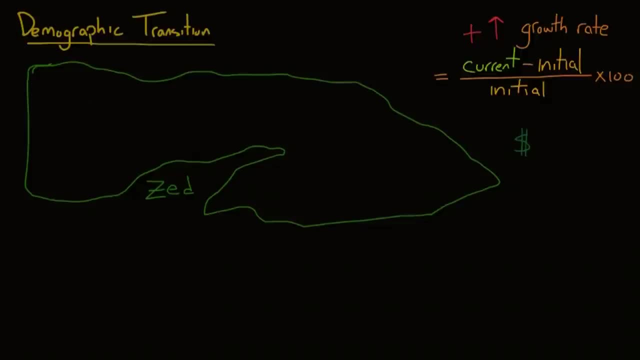 because children can work to help support the family, and sometimes the government even provides incentives to families for each child, like in Japan, where birth rates are very low. Religion also influences population growth because it often promotes large families, which increase the number of people in their faith and encourage a stronger community. 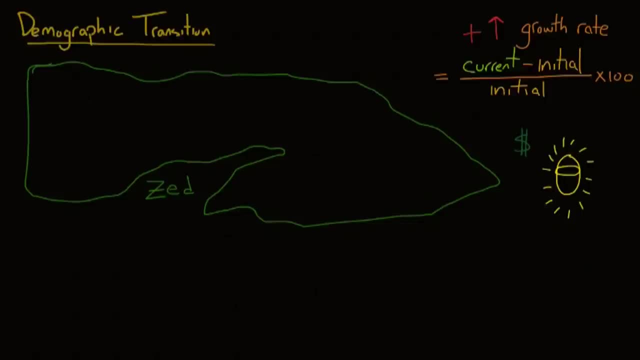 The country's birth rate will even forbid the use of contraceptives by their followers, pretty much ensuring large families, And there are cultural influences that promote large families too. Having children means that a person is passing down their own family's traits and values, and there's a kind of prestige. 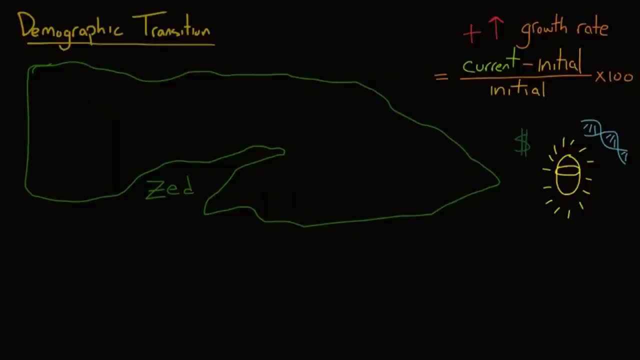 that goes along with having children. OK, now let's dive into the demographic transition model. There are five stages to the demographic transition model. In stage one, a country has high birth rates, often due to limited birth control and the economic benefit of having more people in the family. So the 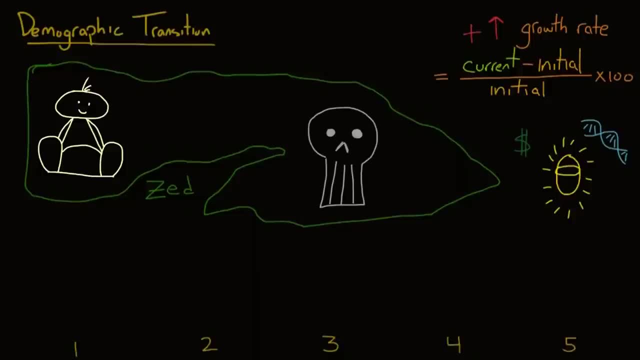 country has more people than the population. On the other hand, that means there are more people to work and they also have high death rates due to poor nutrition or high rates of disease. It is believed that most countries were at stage 1 until the 18th century, when 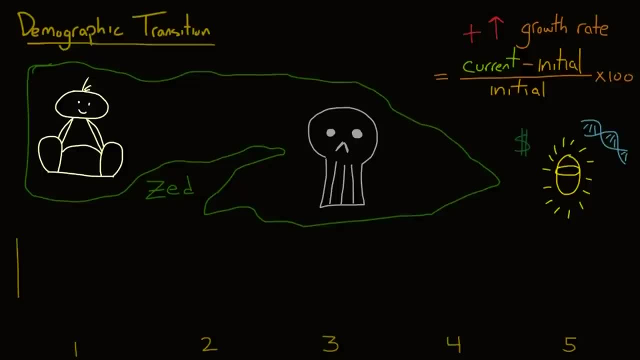 death rates in Western Europe began to fall. You can see this type of population modeled by a high stationary population pyramid with a high birth rate. This pyramid shows the number of people alive in a population, depending on age and gender. As you can see, this stage 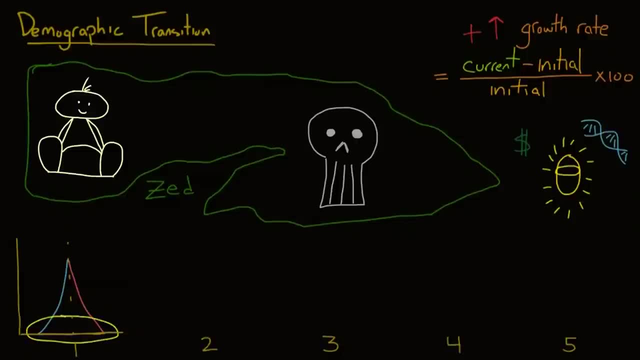 1. stationary population has many births, creating a large young population, as well as many deaths, creating a small older population and keeping the overall population fairly stable. The second stage is seen in the beginnings of a developing country. The population begins to rise as death rates drop because of improvements in health and sanitation and the availability. 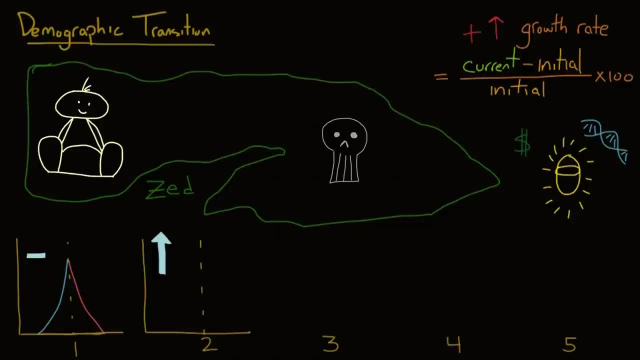 of food. This trend can be seen in Western Europe in the 19th century, after the Industrial Revolution. The birth rates are about the same as they were in stage 1, though, so the overall population begins to grow. This is an early expanding population pyramid. You 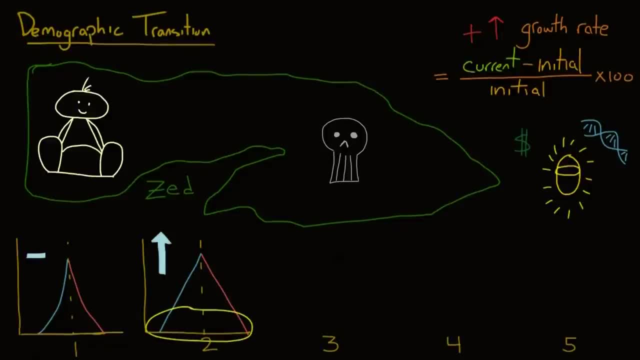 have high birth rates, still see lots of young people, but the death rate is declining, so you have more older people making this nice pyramid shape In stage 3, the death rates continue to drop, but at the same time birth rates also begin to fall because of access. 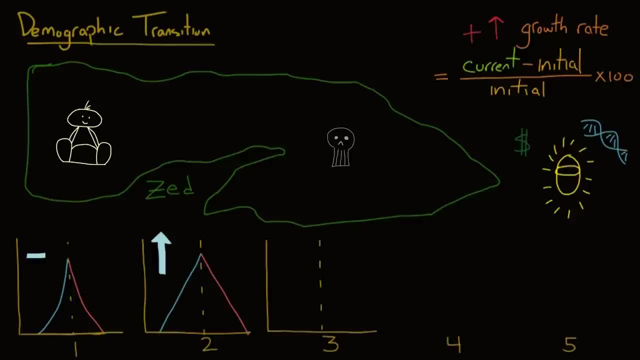 to contraception and a changing social trend towards smaller families. The society is better healthcare and is becoming more industrialized by this point, meaning there are more and fewer childhood deaths and also the kids don't need to work or are not allowed to. 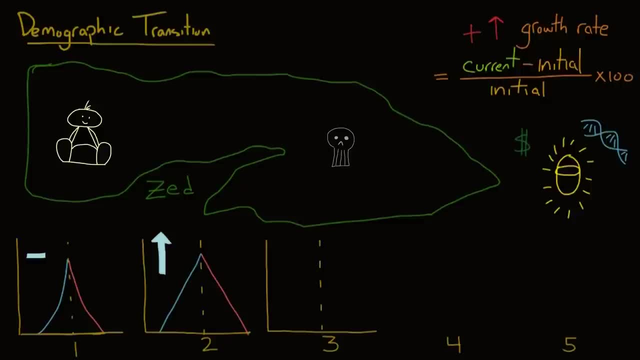 work by law anymore. Having lots of children isn't economically beneficial anymore, as their kids are sent to school rather than working to support the family. Many countries in South America and the Middle East have such declining birth rates. This population is still expanding, but at a slower rate. You can see in this late expanding population. 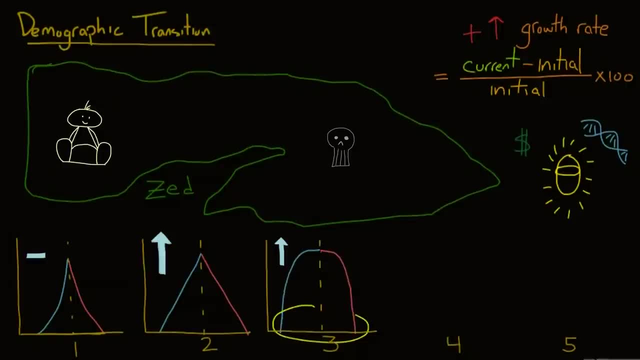 pyramid that as birth rates decline, there are fewer young people and, with the already declining death rates, people are living longer. The second stage is seen in the early 20th century. The population finally stabilizes in stage 4 of the demographic transition model. 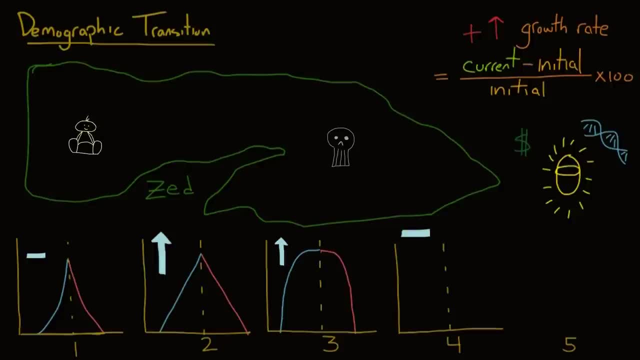 where both birth rates and death rates are low and balance each other out. By this point, the population is rather large because it has been growing up until this point. The low birth rates are due to a combination of improvements in contraception as well as. 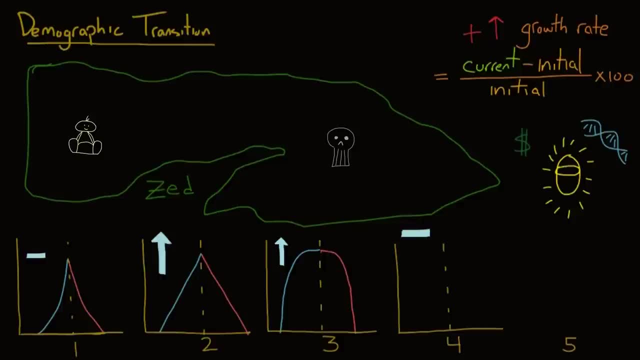 the high percentage of women in the workforce and the fact that many couples choose to focus on careers over having children. Countries like the United States or Australia are in stage 4 right now. The population can be modeled by a low stationary pyramid, with low birth rates and low death rates, as well as a longer life expectancy. 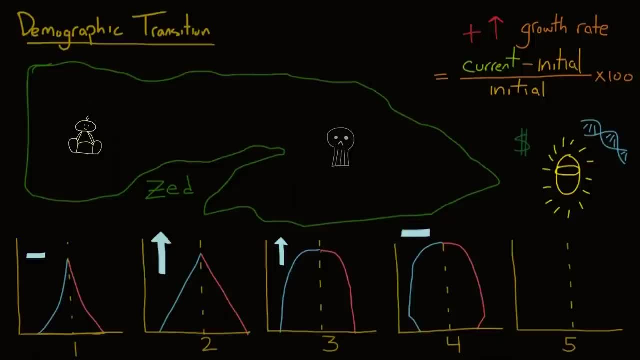 The fifth and final stage is only a speculation. There are a few theories as to what happens next. Some believe that the world population will be forced to stabilize, As the Malthusian theorem suggests. perhaps we will run out of resources and there will be a global food. 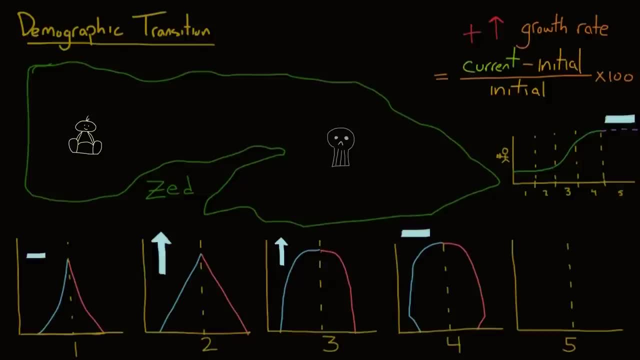 shortage Already. of the more than 7 billion people on our planet, there are about 2.5 billion worldwide who suffer from hunger and malnutrition. The world population continues to increase, but perhaps we won't be able to maintain the natural resources at the rate. 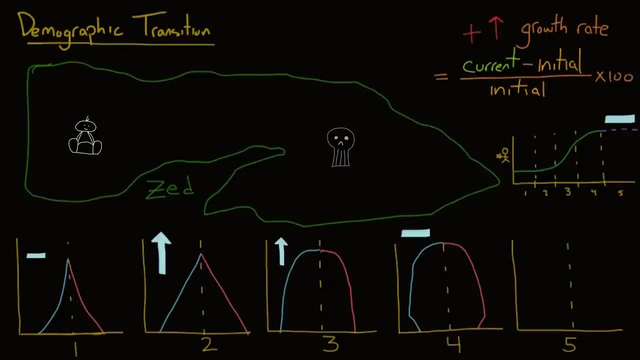 we are going for? how many people live on this planet, which Malthusians believe will lead to a major public health disaster and force the population to remain stable? Or perhaps the population will begin to decrease after it stabilizes, continuing the trend of decreasing?